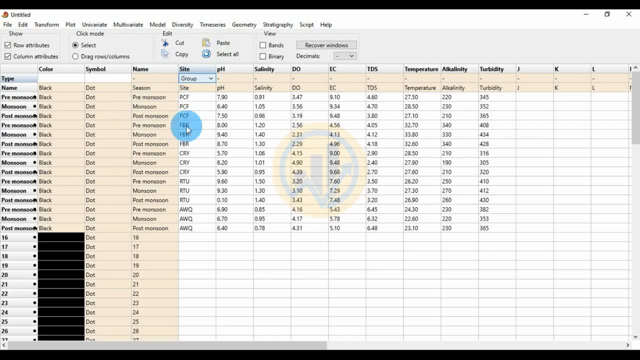 the type of is change to group. Ok, now they change color for the seasonal and the different side. They change color: The first side. for the PCF, they change the AQW color. The three seasonal is the same color, The same side, and the next one is for the PCF. They change. 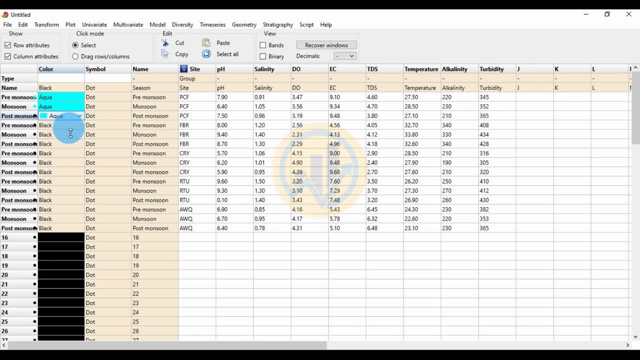 the AQW color. The three seasonal is the same color, The same side and the next one side for the change to color, the FBR, the change color- They are rotated coincidentally together for color inappropriate. And the third one side, another for the change. 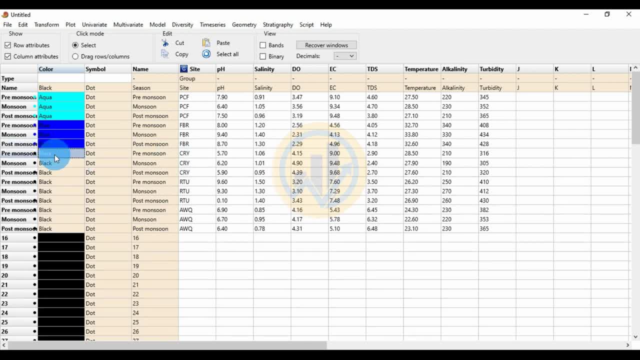 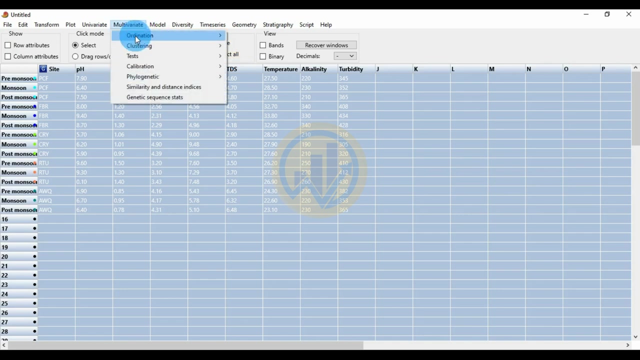 to color. they are rotated too. color Vote and then settle predetermined. The third one, Then fourth, one side for the RTU: Change color. And fifth, one side for the QAW, The QAW, change the color. Ok, Now the unclick for the column attributed and row attributed. checkbox Select the whole. the data Go to the multivariate menu, The ordination. The first one for the principal compound analysis. 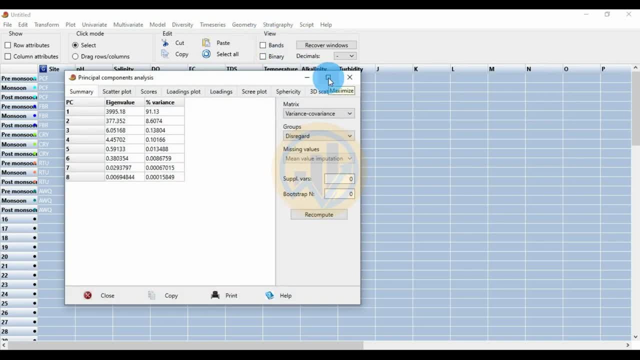 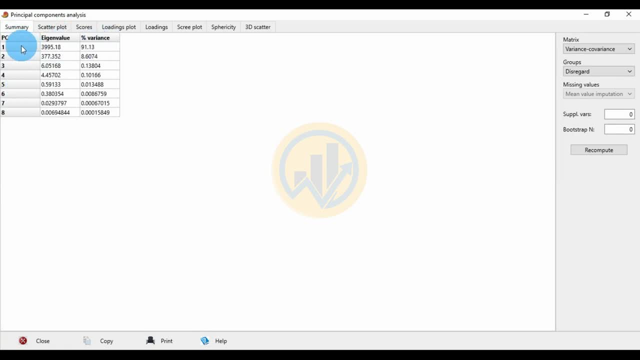 Ok, Open the new tab for the principal compound analysis. The first one tab for the summary: The PC aid value, The ICANN value and percentage of variations: The PC1, the highest value. The PC2 present the ICANN value, The highest percentage of variation. 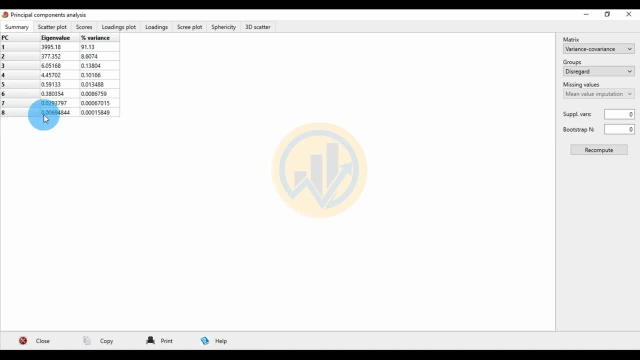 The lowest for the PC aid value, The principal compound analysis aid value And lowest variation, The middle of the fourth PC value, The middle of the fourth PC value And the percentage of variation And the percentage of variation. So that, basically, was the whole analysis. 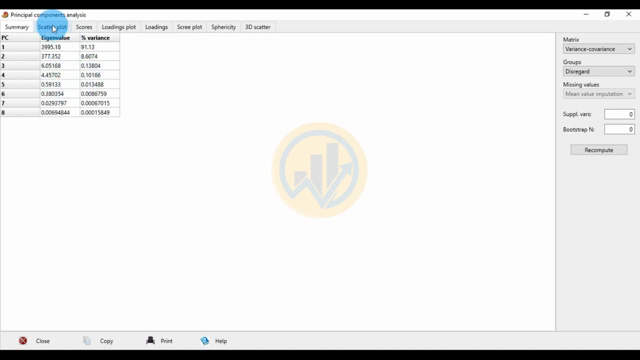 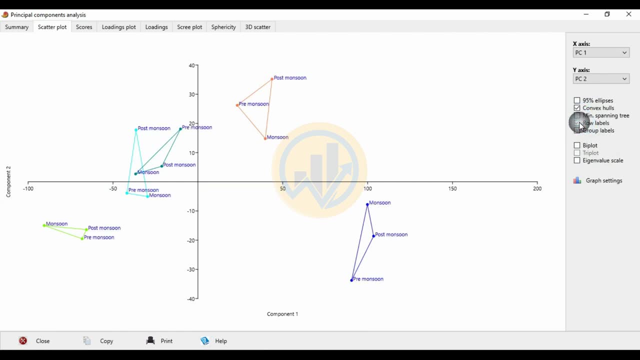 Next one for the scatterplot: The scatterplot. This is a scatterplot for the principal component analysis. They clicked the convex scales And the row label and the group label. The next one for the Baiplat: This B thời to be ghee. 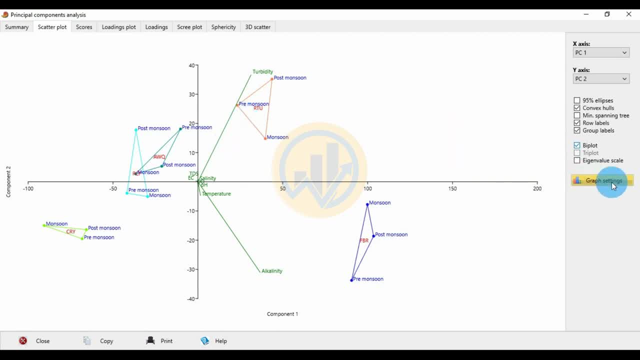 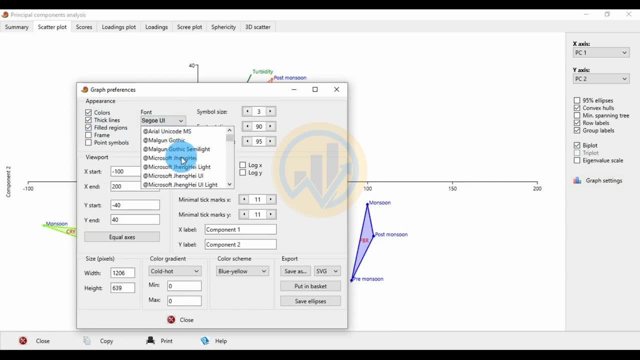 Also for the parameter parameter: system parameters. The water samples are fast. Now go to the crop setting In the field, the check box and the thick, light thick line and fill the region color and change font for the time Roman. okay, the font size is set to all. increase it. okay, then close it. this is for the scatter flat and the principal. 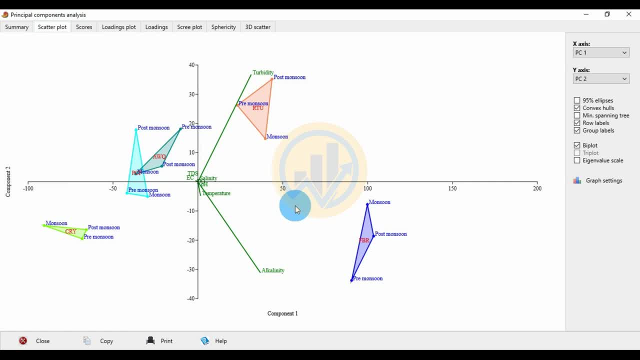 compound analysis, the first one for the PCF group, the PCF, the site locations, the PCF- this is a PCF locations, the principal compound analysis in the PCF first locations. and the pre monsoon: the value, the pre monsoon value, the PC one value. this is a PC one value under. 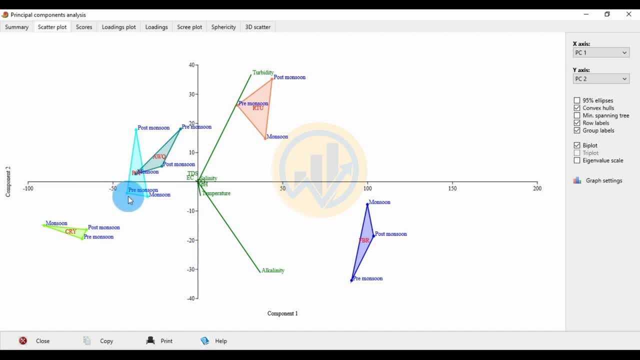 the principal common to value there. this is a pre monsoon. the value minus 41 for the PC one, the minus 41 at same time. the piece to be a PC. to value for the 0 minus 3. this is a minus 3 at the same time. the monsoon, the monsoon, the principal common analysis, is a PC. 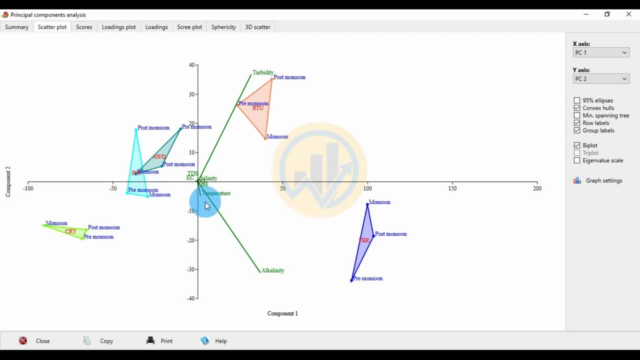 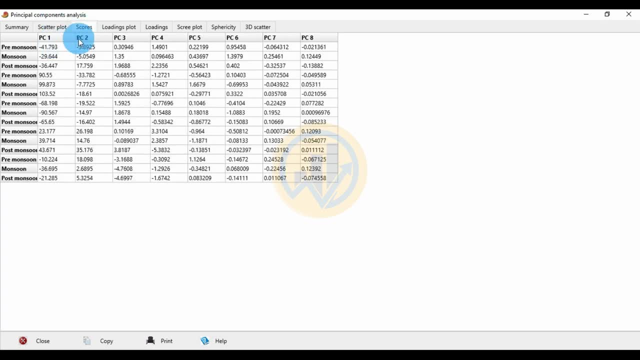 1 value minus 29 are the PC 2 values here: 0.5, 0.05. this is the table. percent in the score value. this is a PC 1, PC 2, PC 3, PC 4, PC 5, PC, PC 7. out of the PC 8 value, the percent and the whole the data in: 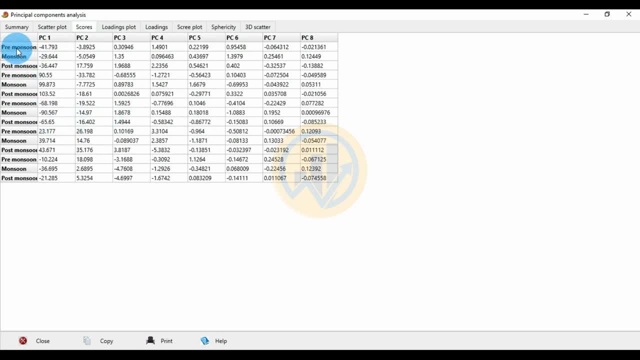 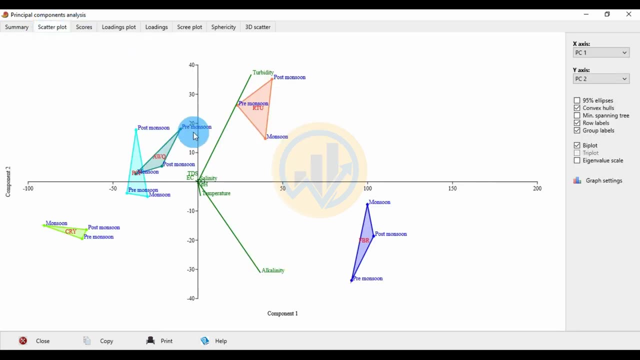 the table: the pre monsoon, monsoon, post monsoon. the first three, the differences in the group, the location, the PCF. the next one for the pre monsoon, post monsoon, the monsoon is a three different seasonal. in the second one for the FBR group: go to the scatter plant. the next one for the 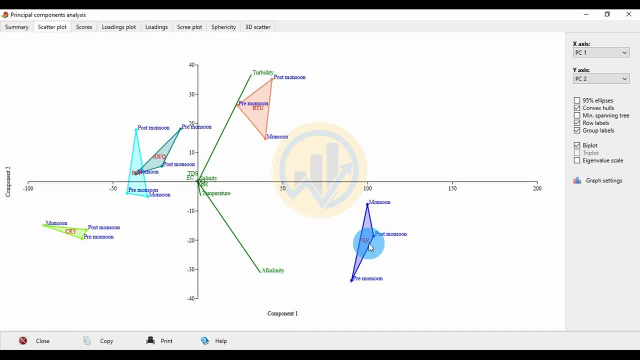 FBR group- this is a second one for the FBR. the locations- this is a first. the seasonal for the pre monsoon, the PC one value for the 19.55. this is a positive value, at the same time the negative. for the PC 2 values here minus 33 are the monsoon period. the value PC 1, the positive value from the. 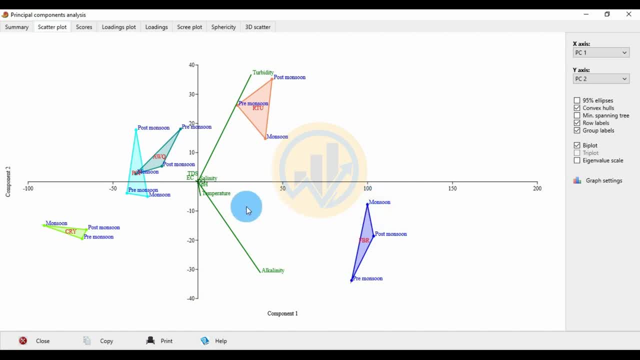 99.87 are the PC 2 value for the minus 7.77 are the post monsoon for the third seasonal. the FB are the group, the positive value for the hundred and three point fifty two with the PC one at the same time. the minus eighteen point sixty one with the principal common to value then third one. 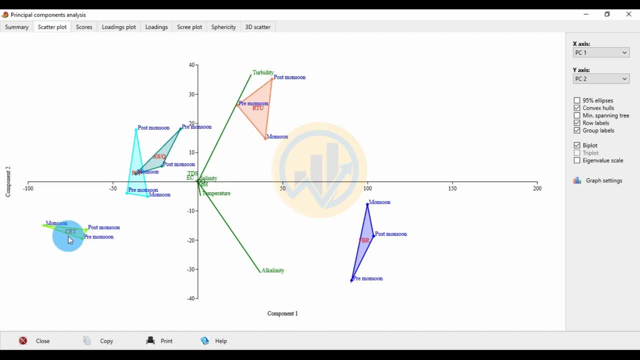 C? R Y. this is a C? R Y, the C? R Y, the pre monsoon. the pre monsoon value, the PC one value minus 68.19, the minus 68 point. the PC one is a minus 60.1, a minus 68.8, 19. at the same time, the PC 2 values are minus 19.52. 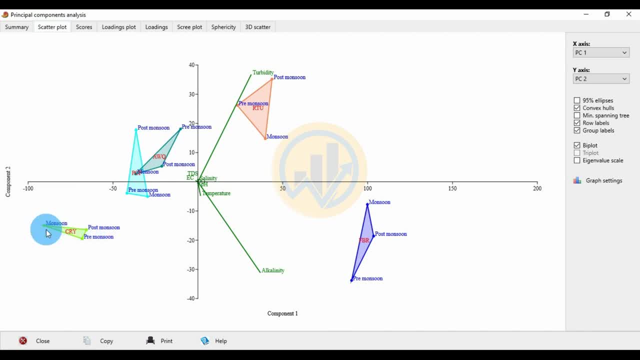 the second one for the monsoon season: the PC one value for the minus 95.56. at the same time the PC 2 values here minus 14.97. the third one, for the post monsoon, is a principal compound analysis: PC wonderful value minus 65.56. at the same time, the PC 2 values here minus 16.48. this is a principal. 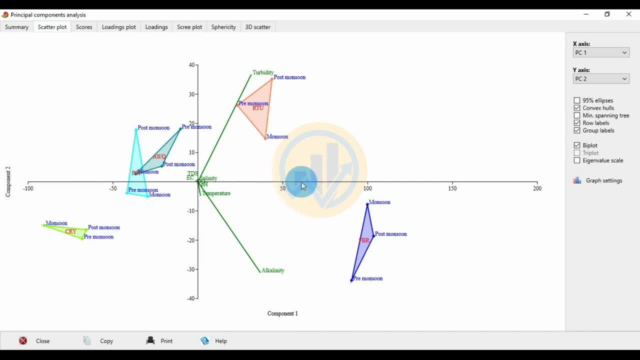 two: this is principal compound analysis. one: this is a principal common analysis. one: this is a principal components two. the next one group are the RTU. the RTU, the free monsoon period, the pre-man's in the value for the positive value in the PC one under PC two, the pre-month in the PC one. we're say twenty three point seventy at the same time. 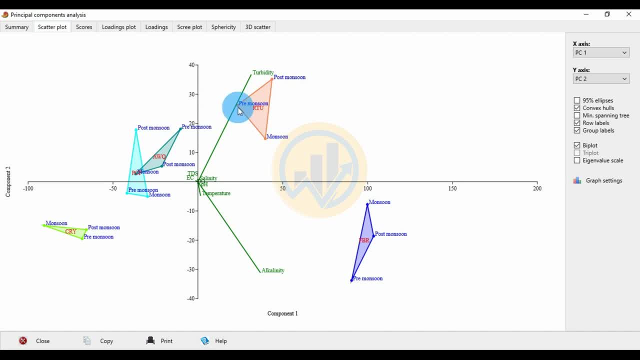 for the pre-monsoon, the at the same time, the PC2 value is here 20.19. okay, the next one for the RTV value: monsoon period: the monsoon period, the monsoon period value 19.39.71, the PC1 value or the PC2 value 14.76, and the post. 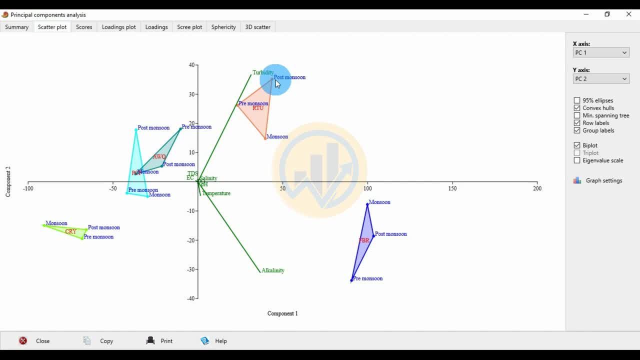 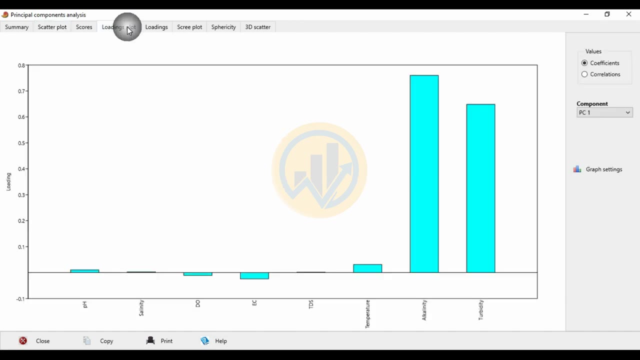 monsoon, the PC1 value the 43.671. at same time the RTU in the PC2 value 35.176. then next one for the loading plan, the loading plus the principal componently 8 component, the PC1, PC2 and PC3. 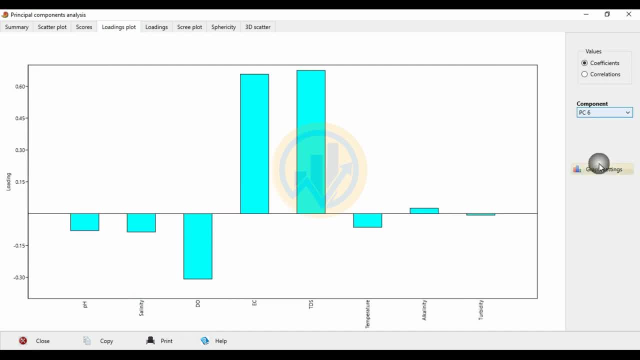 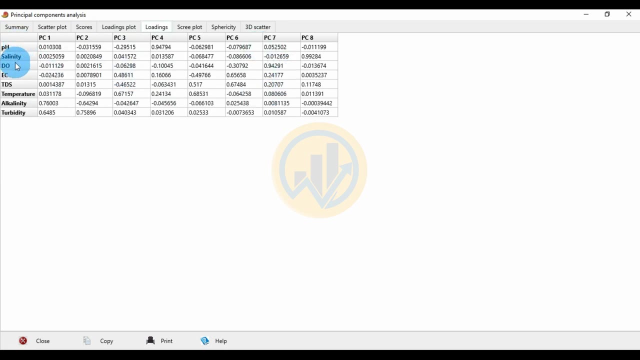 and the PC4, PC6 and PC7 and the PC8. the worst component for the PC1. this value presented in the loading chart in the table. the next one, the, the water parameter for the pH, salinity, DO, EC, DDS, temperature and the terminity, the PC1 value presented in the positive. the salinity also positive. 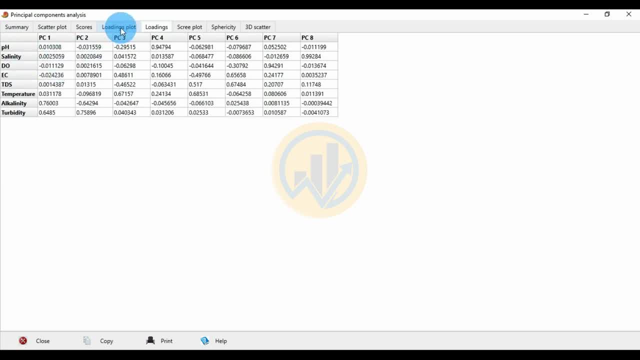 DO is a negative for the 0.011. the 0.0 level is a DC DO value. the next one for the EC also. 0.011. the 0.0 level is a DC DO value, the next one for the EC also. 0.011. the next one for the EC also. 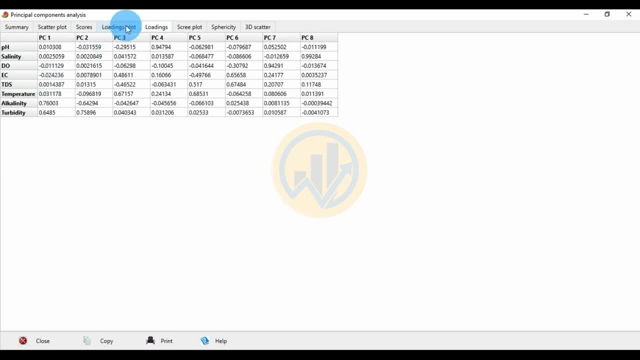 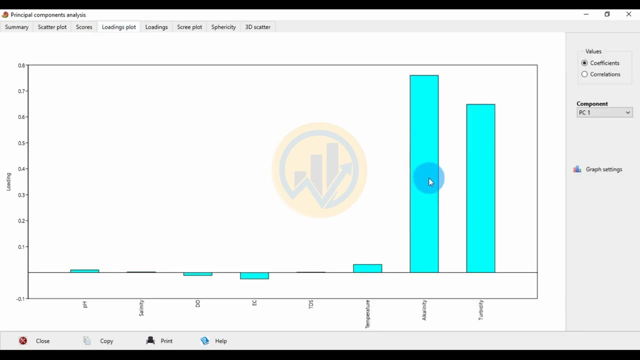 0.01.. THE TERMINITY karış not below 0.1.. DOWN, in this case it is positive VALUE to ground 4.1.. at the next one, since the top NONむ2, it was really Andrew- 4 bottom than F square exclusively common, is the third, which was least from my. 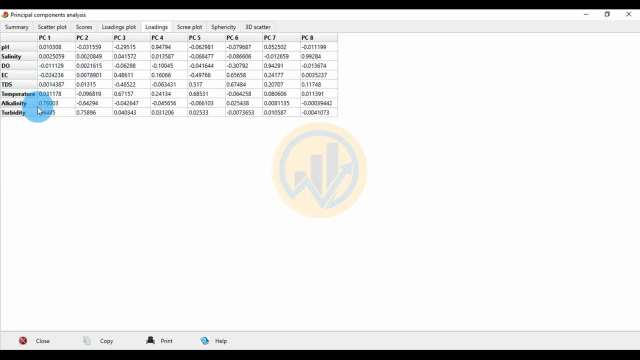 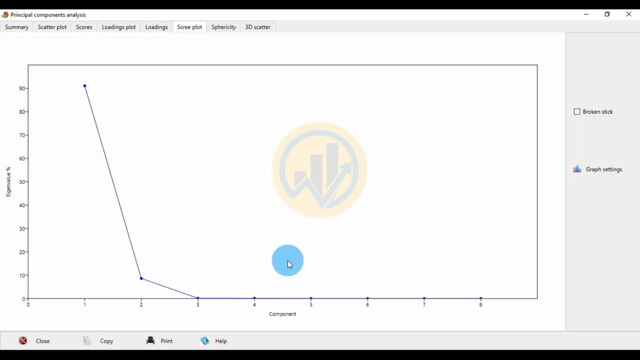 наверное scar blood, the scar blood, the v1, the principal compound analysis. the principal compound one and two is the highest value presented under three, four, five, six. there the average values. the next one for the scalping, the badless spirituality test, the not supported for the grouping principal. 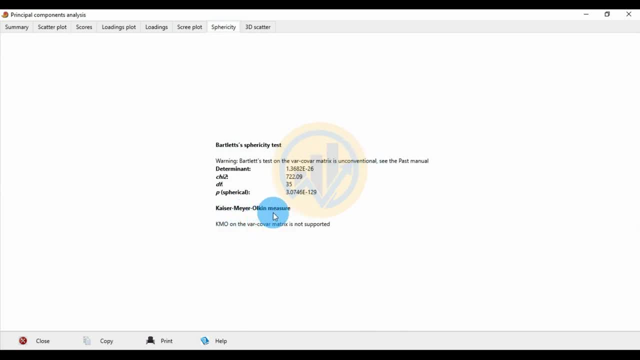 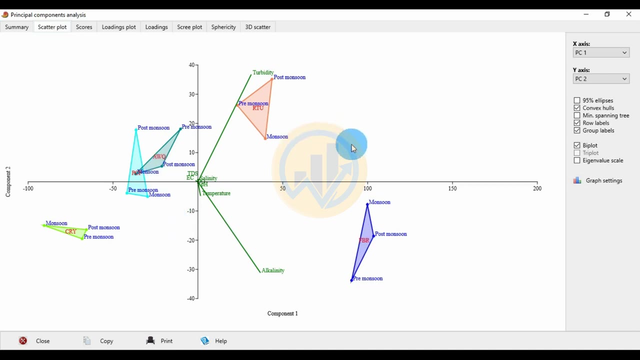 compound analysis. in the test, the high square, my all-kind measure, the test, also the not supported for the grouping. principal compound analysis. the next one's tab for the 3d scatterplot in the principal compound analysis. okay, this is a main chart for the principal compound analysis. 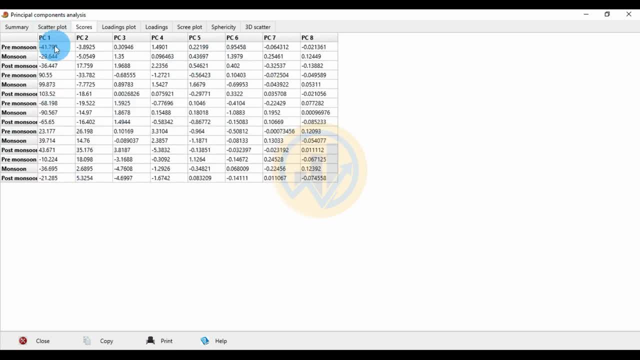 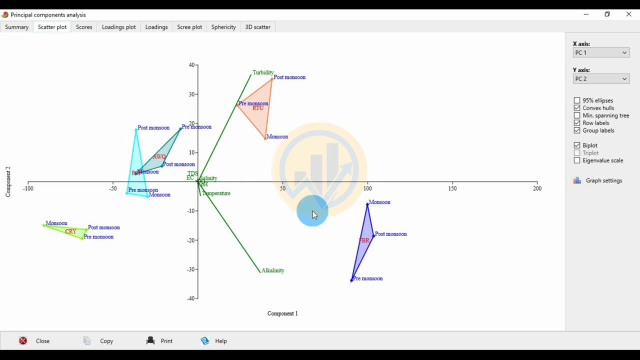 and the main value. this is a table for the principal compound analysis. if you like our videos, please like and subscribe to our channels. thank you for watching this video you.